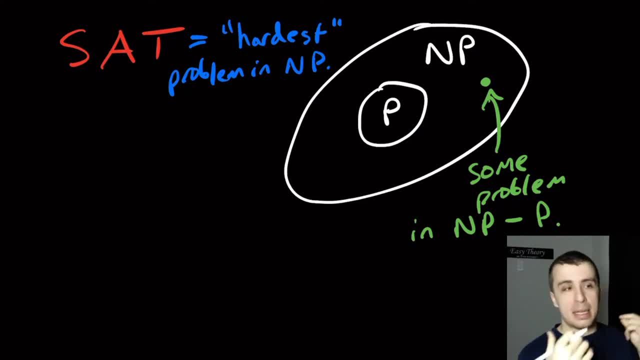 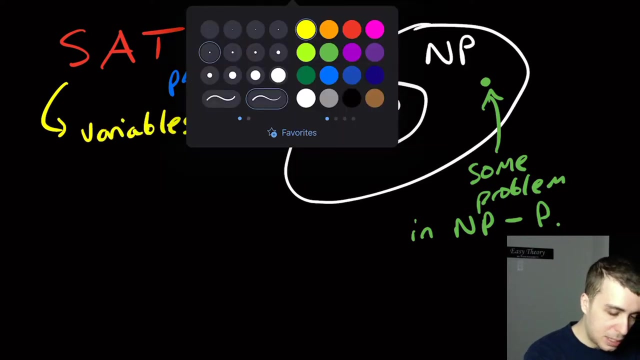 the reason we want to do Boolean formulas is that they can encode a whole host of problems that researchers are working on, and practical problems too. So how do you actually make a Boolean formula? So we have variables, So a SAT instance has variables in it, And these are Boolean. 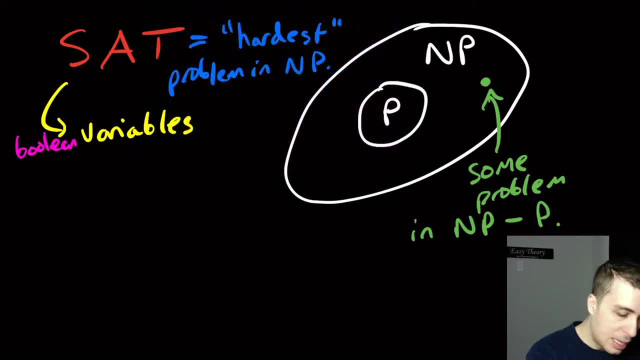 variables, I should say, And so of course we have a Boolean formula, And we have a Boolean formula, And so of course they can. let's call them, let's say x1,, x2,, x3, up to let's say xm. It. 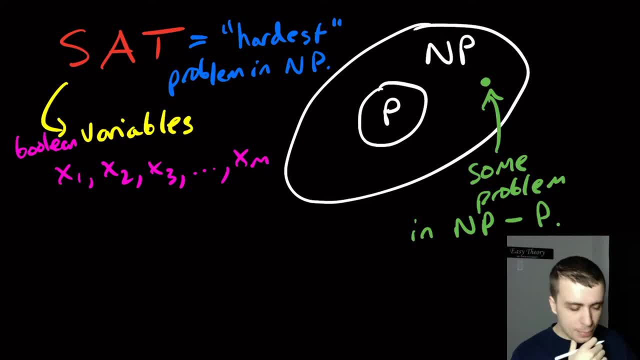 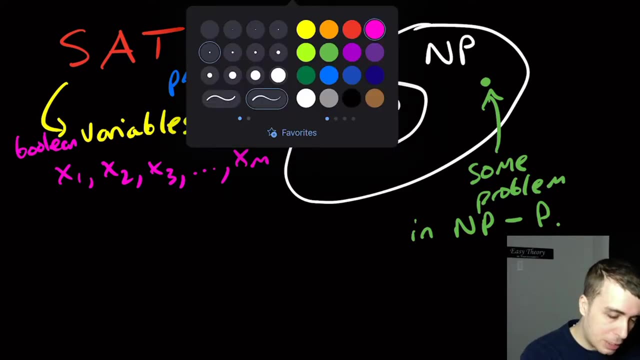 doesn't really matter. It doesn't matter what you call them. In fact, in subsequent videos I'm going to use different letters for different purposes here. So x1 up to xm, these are the variables here, So we can combine these using some operations. So not only does it have variables, but it also 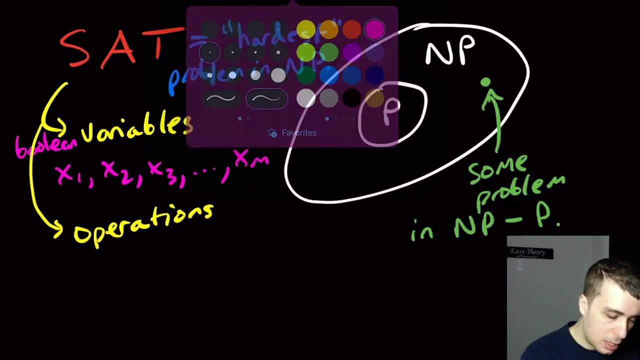 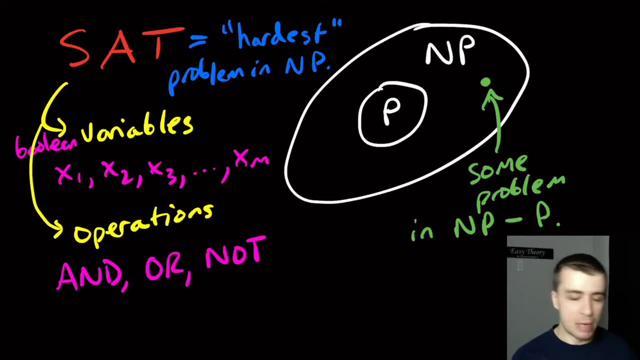 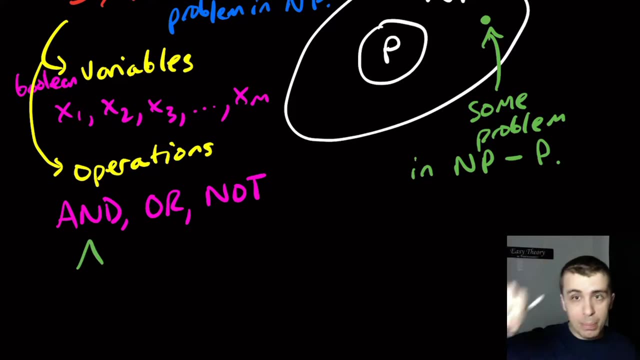 has variables, And the ones that we're going to use are AND, OR and NOT. So those are the three operations we can work with. You can use others in some other context. So the way that we encode AND is: with a little wedge symbol. It looks like an upside down V, OR looks like an actual V And. 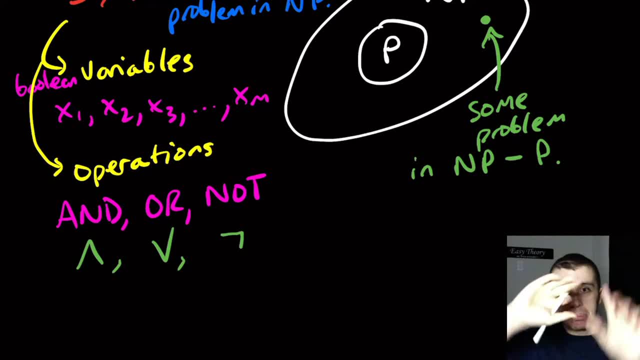 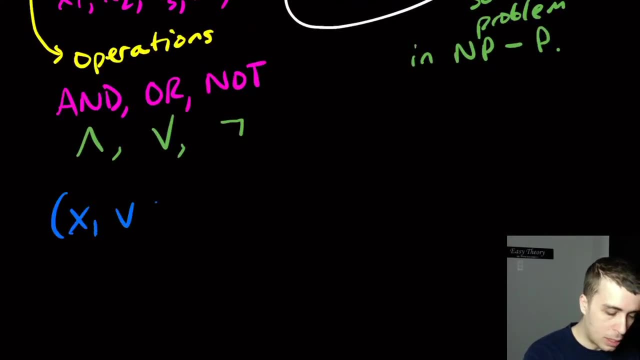 NOT has this little sideways backwards, L-shaped thing. How are we going to combine these? Well, we can combine them in any way that we want. So we could say, for example, x1 OR x2, a complement OR x3, and then, AND Maybe we have x1 AND x1 bar. 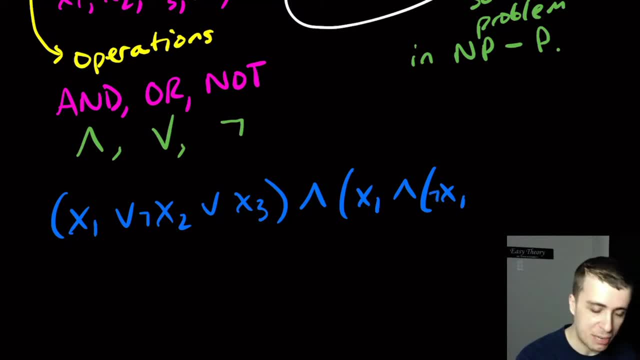 Sometimes we put the bar upstairs, but I'm going to put it on the side for now. OR x2.. So we can have nesting if we want to, We can have single elements on their own, And then we can have an OR on the outside if we want to, even though I should probably put parentheses. 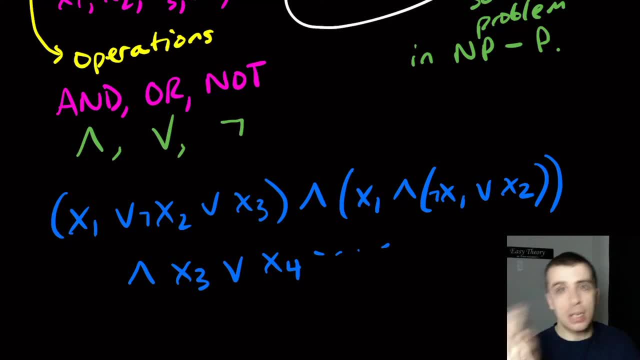 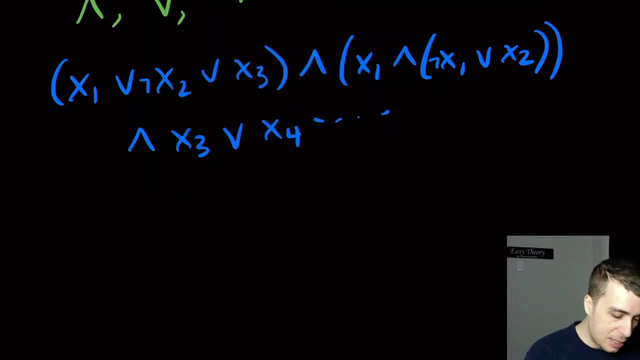 around it, And then we can just obviously continue like this, So we can combine these operations in any way that we want. OK, So then we say that let's call this formula phi. I know it looks like the empty set. Maybe I should use it differently. 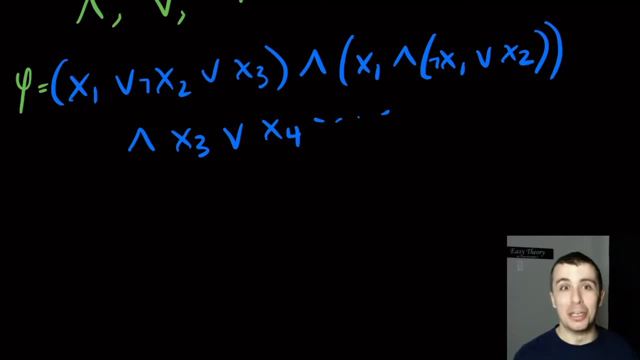 It's pretty simple. Let's do psi, which is close, But it's a psi, not a phi. So we say that this psi is satisfiable. I should be able to spell this by now. It's satisfiable if we can assign. 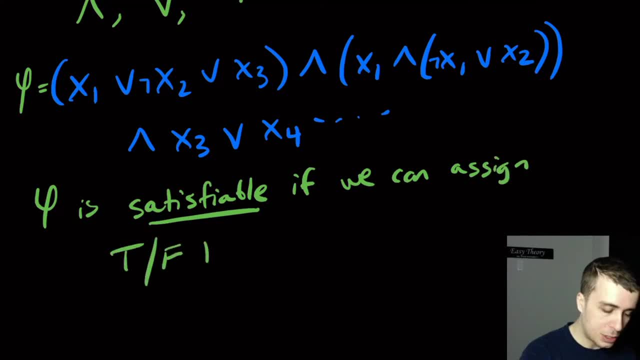 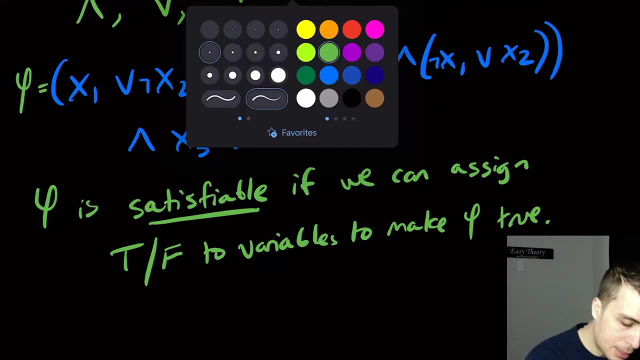 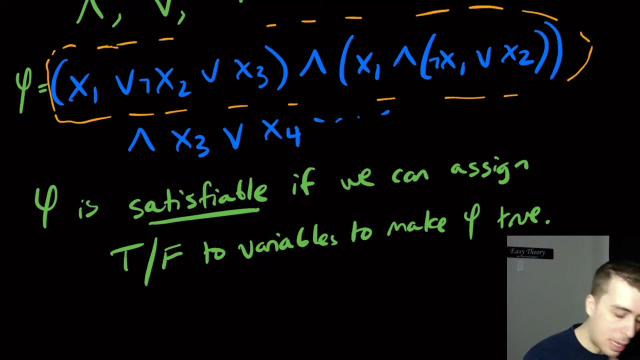 a true or false to variables to make psi true or evaluate to true. So let's look at, let's say, let's look at this first part right here. So let's look at this part right here. So I want to know whether just that first part, 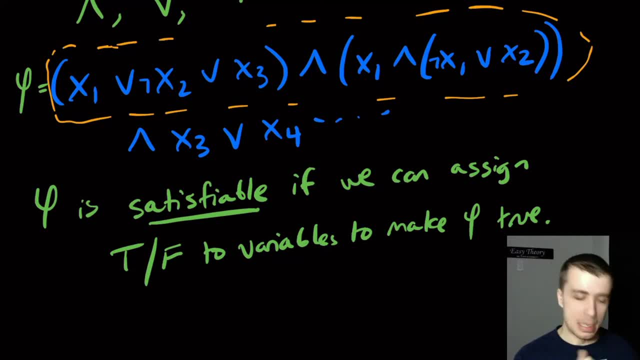 ignore the second part under it whether that part is satisfiable. So if this thing is satisfiable, then by the rules of Boolean logic, because of this, and in the middle it must be that this left-hand side is evaluates to true and this right-hand. 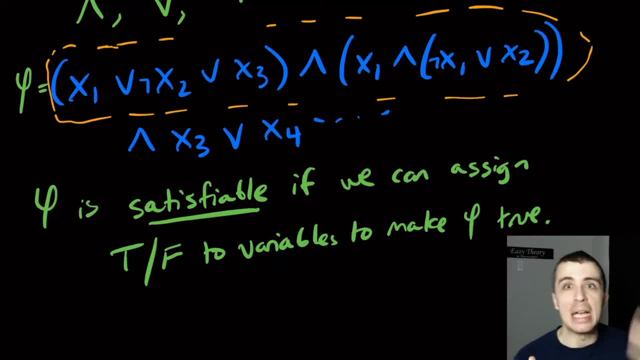 side evaluates to true, Because if one of them is false, something and false is false. So what we can do here is we can say, oh OK, we got a bunch of ors right here, So that means any one of these can. 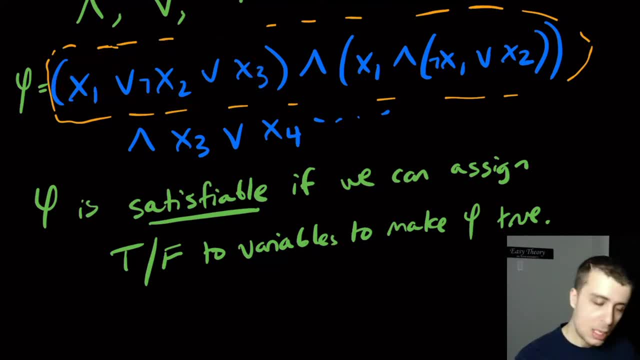 be set to true, And then this left side is true. But note that we have multiple copies of the same variable, So we got to be a little bit careful. So then this right-hand side can be set to true, And then this left-hand side. we got an and right here, So that means that both of these have to be. 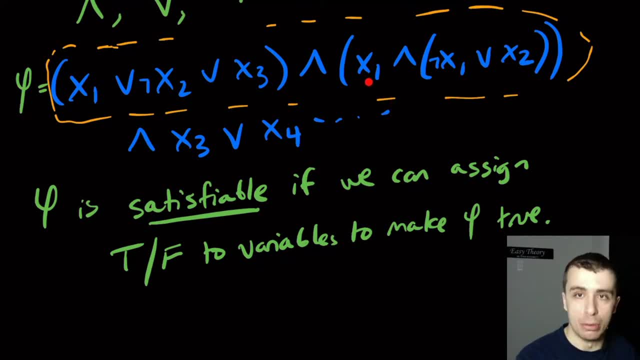 true, which means that x1 has to be true because it's on its own. So if we so we know that x1 has to be true if the formula is satisfiable. If it's not, then it doesn't matter. So x1 has to be true. 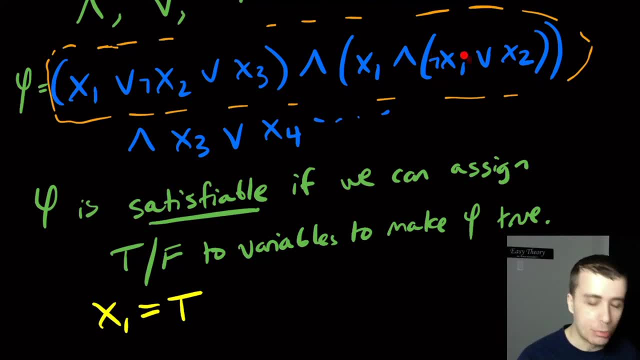 So then over here we have a not x1.. So that is false. So, for this part right here to be true, so then. so then this part is true, This part is true. So therefore, the whole right side is true. 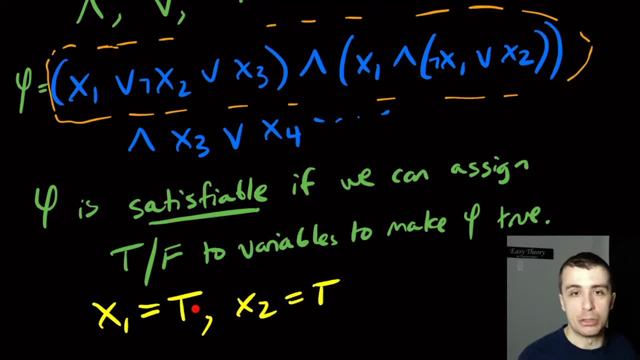 And for this part, we have x1 already set to true by this, So it doesn't matter what x3 is, So we can have x3, be any of the two, And so therefore you can assign this true or false, It doesn't. 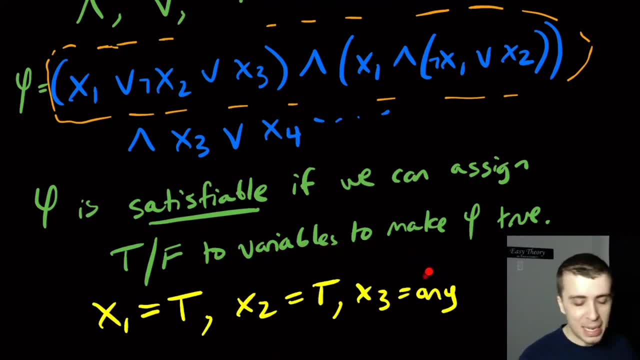 matter. So by this assignment, or pick any assignment for x3, then this formula is set, It can evaluate to true. now, Of course, I could choose a different set of assignments here and then maybe the formula evaluates to false, And so it's not the case of whether it. 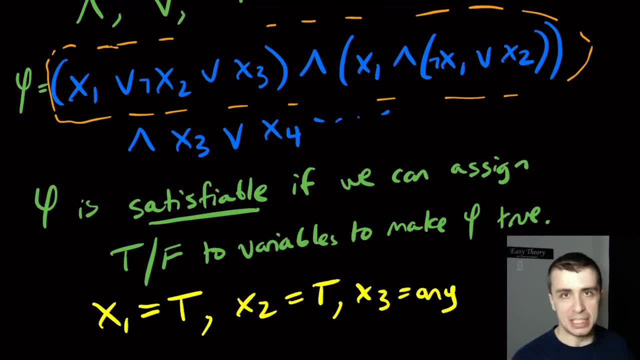 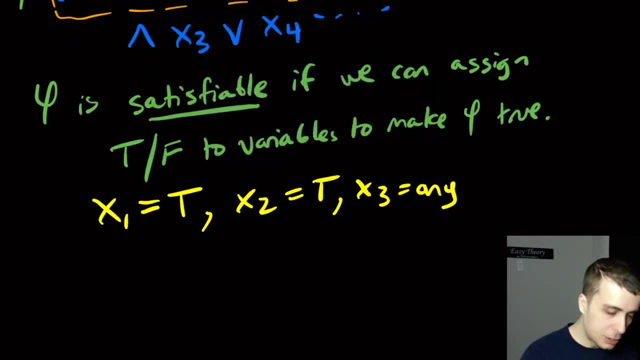 can evaluate to false. I'm wondering whether there is any way to set it to true. So there are different notions of of this. So it's not. sometimes we don't care about whether it's just satisfiable. We want a stronger condition. Sometimes we don't care about whether it's. 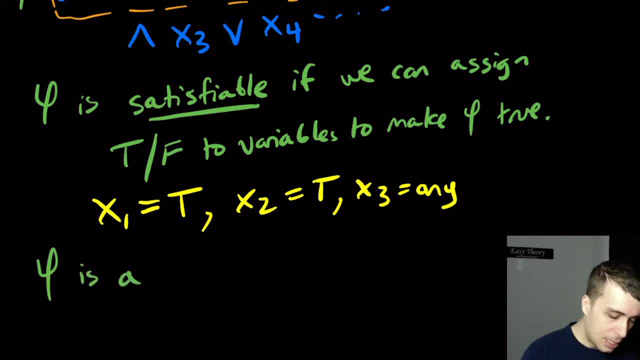 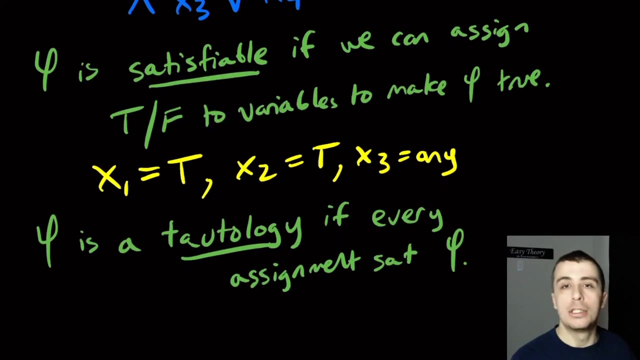 going to be true or not. So in this case we say that psi is a tautology if every assignment satisfies it. Okay. So here we just wonder if there's any assignment that causes the formula to be true. In tautology we worry about whether every single assignment will satisfy the the 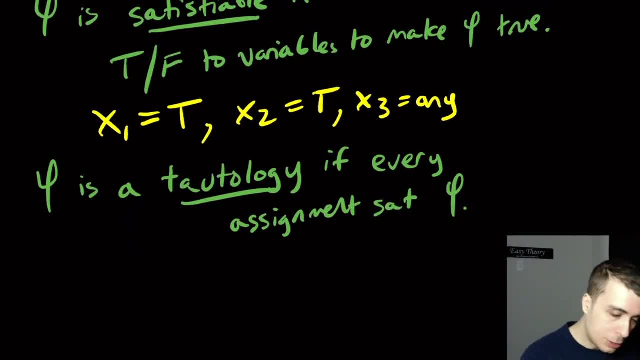 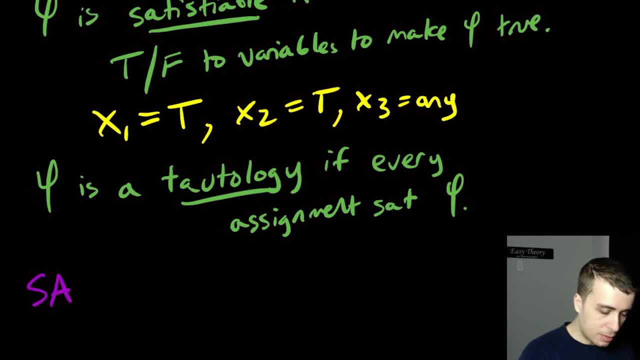 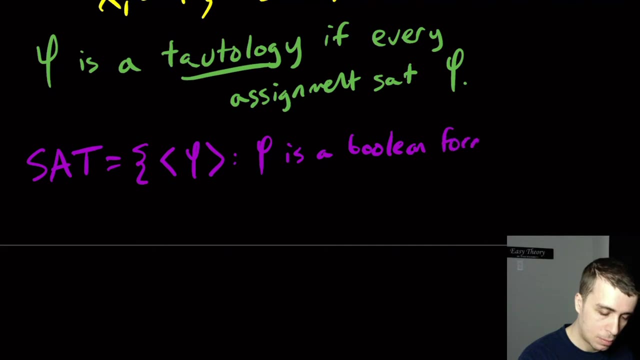 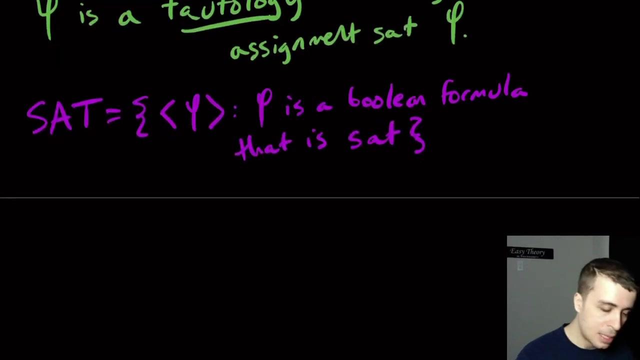 and I'm not going to do now, is that we're going to look at some language, sat, which is the encoding of any formula, so psi. So here we have that psi is a Boolean formula. that is satisfiable. I'll just abbreviate it: it's a sat. So one thing that we're going to prove: 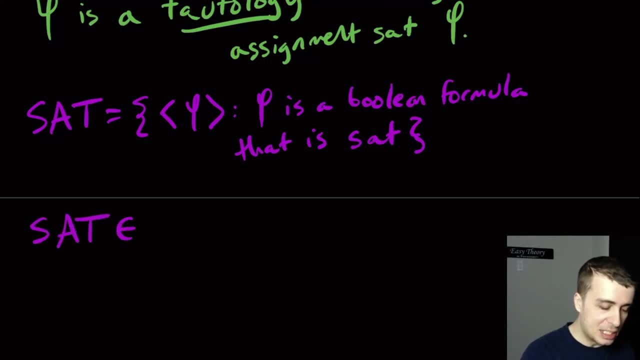 and it takes a long time to prove- is that sat is in p if, and only if, p equals np. so that's the notion of hardest problem that we're going to work with, and we're going to talk about things called np, completeness and other things. so what? this means that if it is in p, then everything.